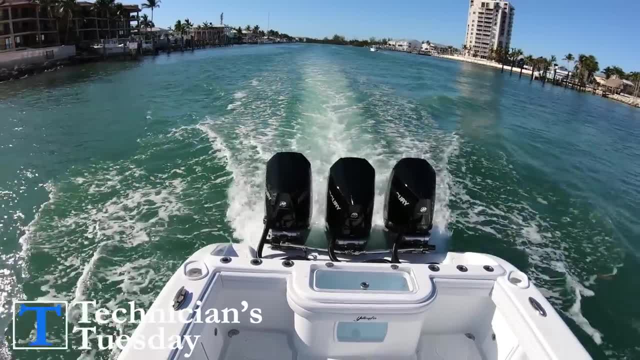 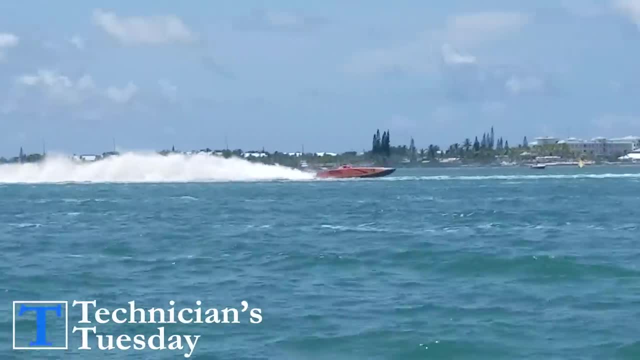 wide-open throttle speed we will be getting. It's important to note that we are talking about the average recreational boating and fishing application here. We aren't talking about racing, though the physics don't change, there are way more variables to consider for racing than what we are going to. 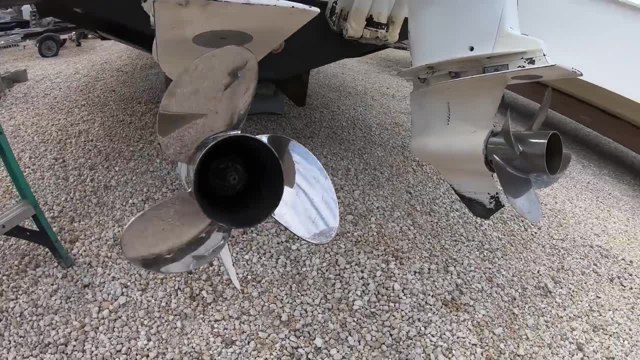 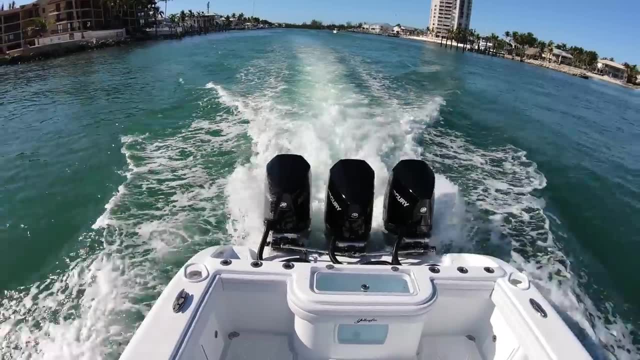 talk about here today. For us, if we go from a three blade to a four blade without changing the diameter or the pitch of the prop, we will lose top-end speed. What we will be gaining, though, is our whole shot: The time it takes to get the boat out of the water. 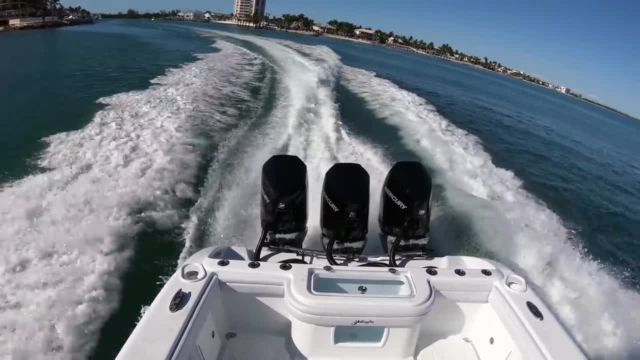 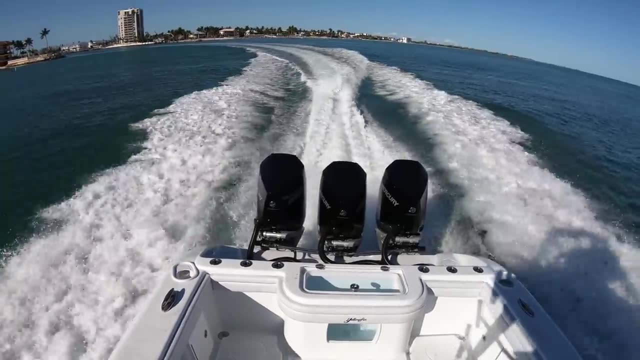 will be way quicker because we have that extra blade which gives us more grip from the prop to the water. With that extra grip we also gain better control and handling. Understanding these things are the base foundation for us to begin the propping procedure to get the right prop for your. 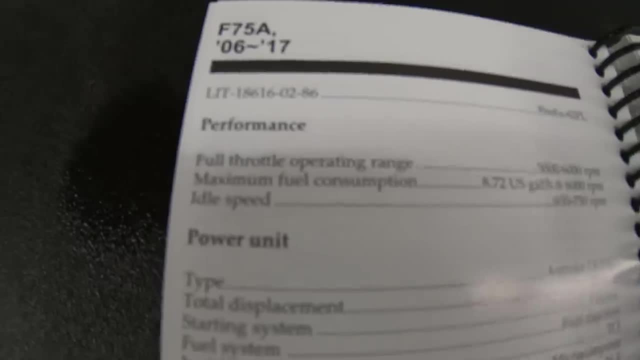 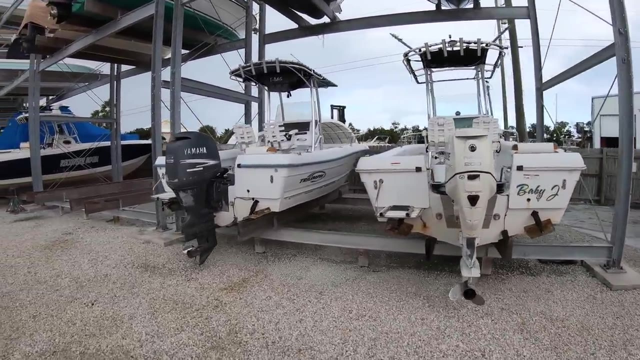 boat. Now each engine is going to have a top-end wide-open throttle RPM range. Each engine that has been manufactured in the last 20 years is also going to have what is called a rev limiter. The rev limiter is going to stop the engine. from going over a certain amount of RPMs. We'll take a Verado for the first example. The RPM range for most Verados is 5800 to 6400 RPMs and the rev limiter is set to 6500.. On a 300 horsepower Yamaha. 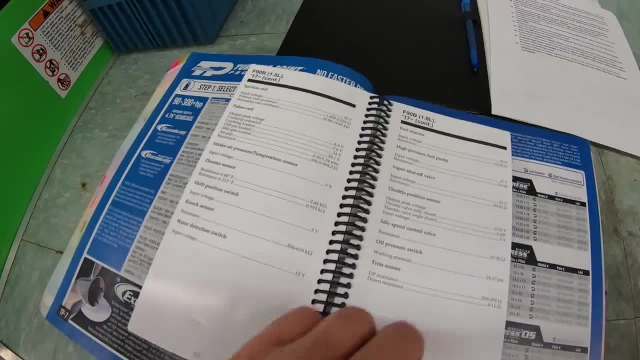 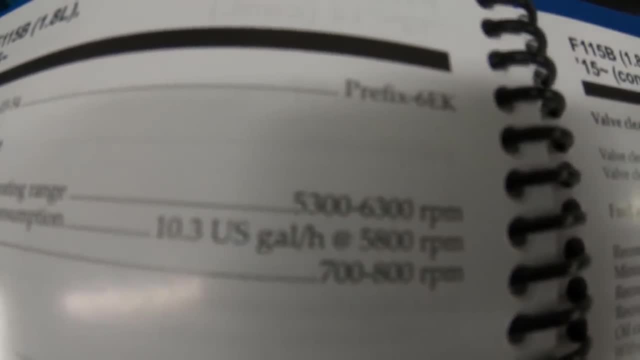 the RPM range is 5000 to 6000 RPMs and the rev limiter is set to 6300.. The rev limiter setting isn't as important to know. It's the RPM range of your engine that you need to know about. If we put a small diameter prop on an engine with a 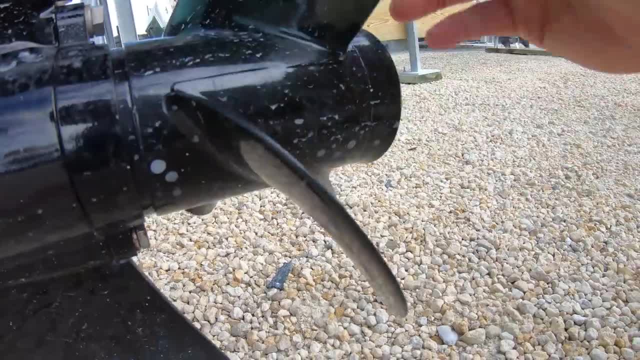 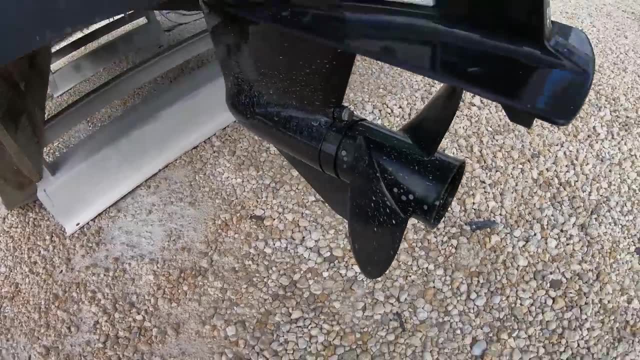 low pitch, the chances are that the power of the engine is going to power through the ability of the propeller to grip the water and push the boat. This results in the engine RPMs going above the specs and hitting the rev limiter. It's 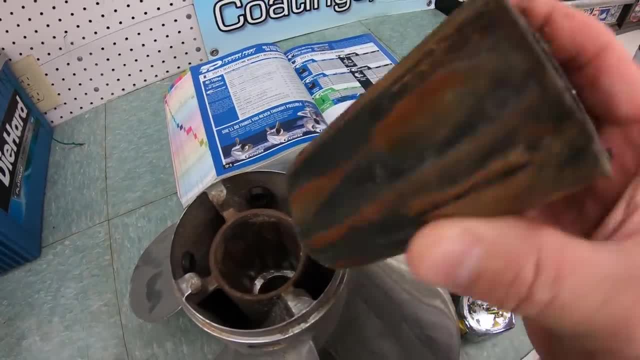 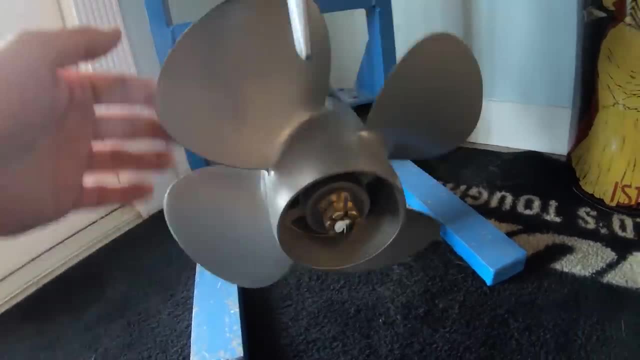 exactly like what happens when the prop hub gets spun. For all of you that have experienced spinning a hub before, you can remember what that's like. On the opposite end of the spectrum, though, if we put a prop with too big of a diameter, 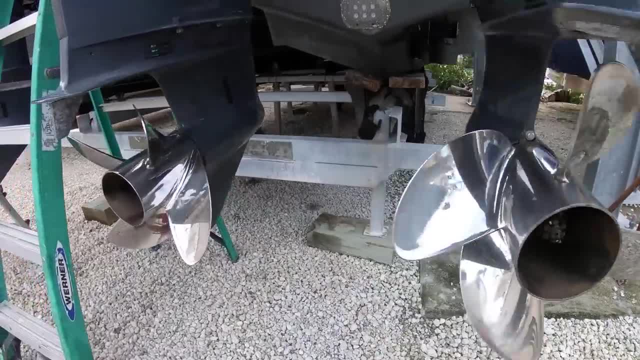 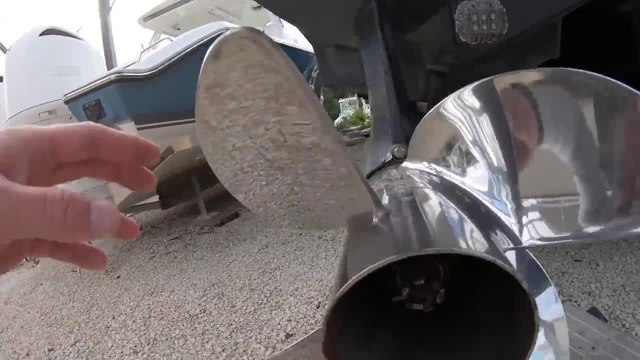 and pitch on, then the engine won't have enough power to spin the propeller up to the right RPM range, causing the engine to never get to wide-open throttle and, if ran like this for a long period of time, can eventually wear out internal. 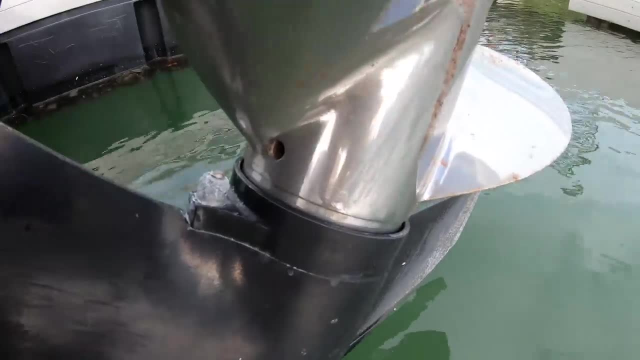 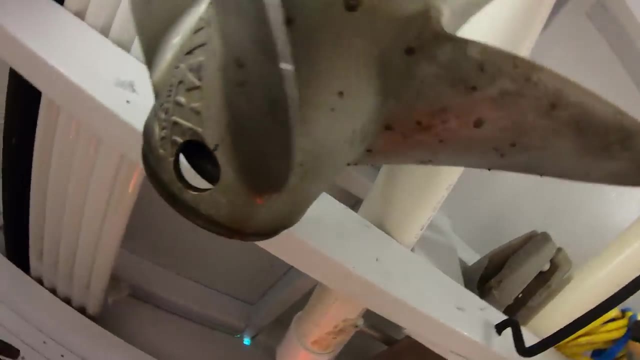 components of the engine prematurely. There are ways to get propeller to turn up higher, though without changing the prop. This is done by venting the propeller. Some propellers have venting holes already on them towards the bottom of the prop. These holes can either be plugged or have the plugs taken out of. 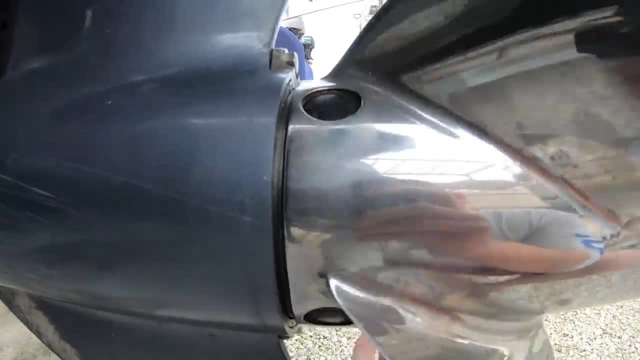 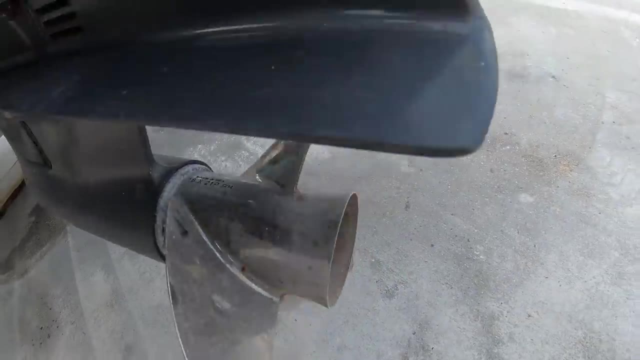 them. What this does is allows water to flow through the prop without having to be pushed off of the blades of the propeller, creating force against the prop. This is useful in a wide range of applications, but we still need to talk about how to properly choose the correct prop for the boat. 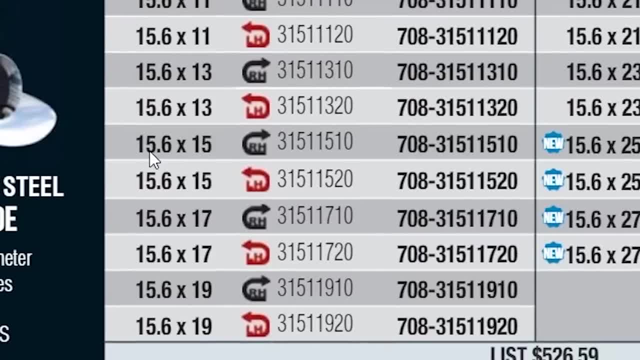 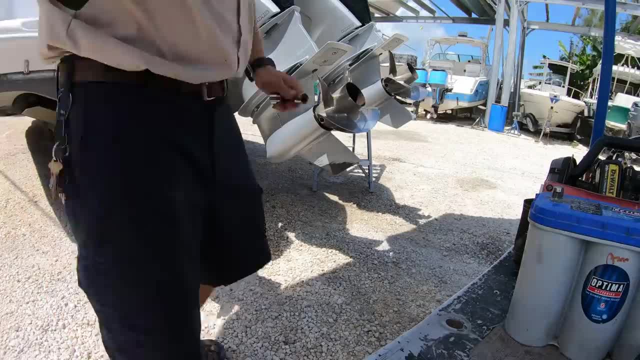 We know about the RPM ranges, the pitches and the diameters of the prop, as well as the ability to vent the prop and go from three to four blades or vice versa, But actually propping out the boat is a process of trial, plain and simple. We 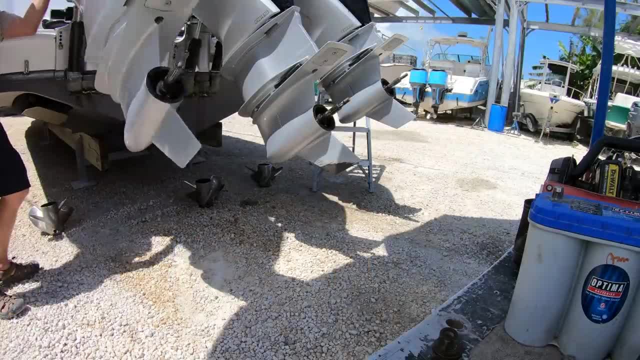 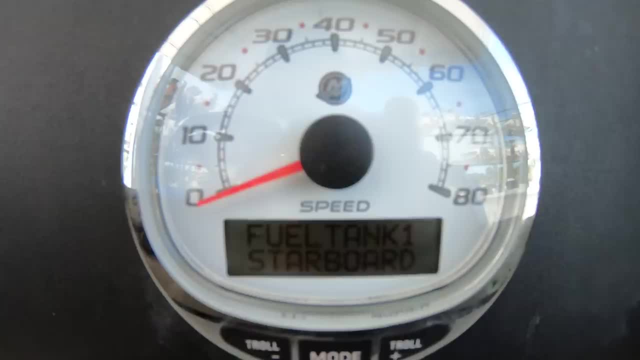 have to make an educated guess of a prop to start with, take the boat out and try it, then go from there. Before doing anything, though, the conditions of the boat make a huge difference, Things like the amount of fuel in the tank, how many? 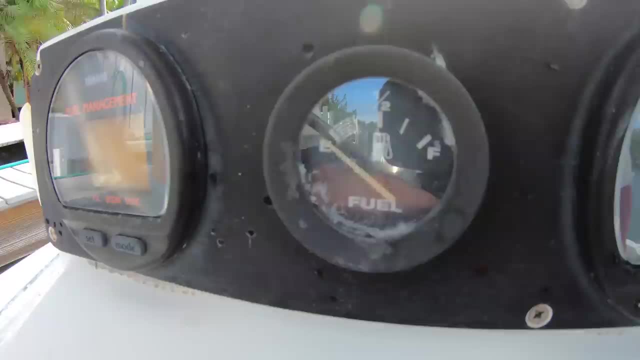 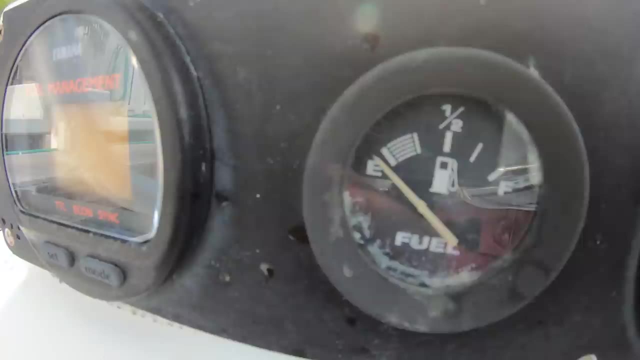 people are on board and what kind of gear we're using. You can prop out a boat with an eighth of a tank of gas. with just you on the boat, The RPM may come out correctly, but when it comes time to use the boat normally, it will definitely. 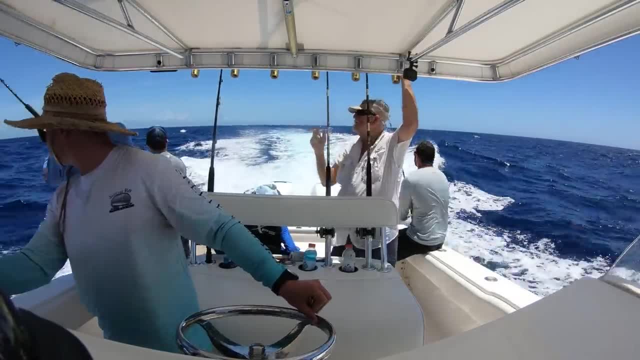 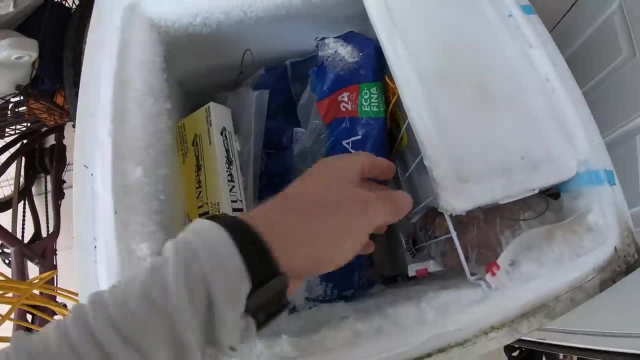 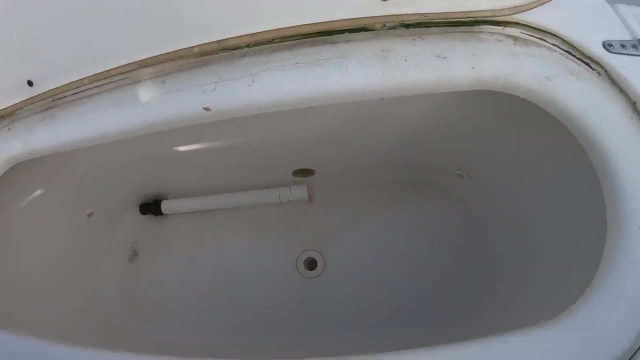 be different. That is because four adults weighing 200 pounds a piece, 100 gallons of fuel weighing 600 pounds, two coolers full of ice, food, drinks and bait weighing about 150 pounds, eight rods and reels, the live well full of bait and water being roughly 250 pounds Now. 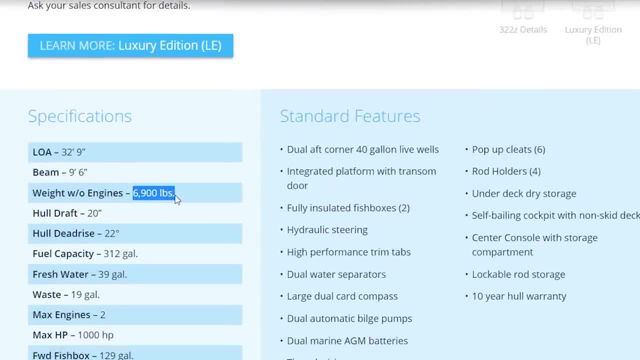 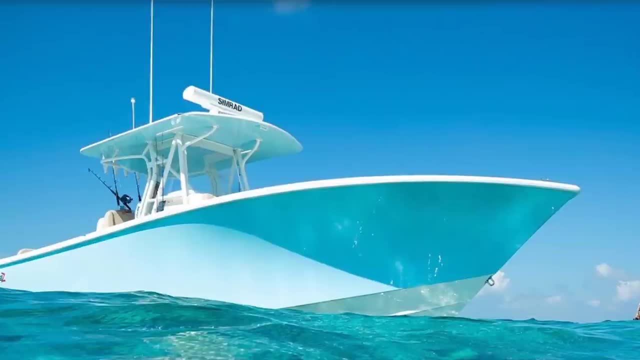 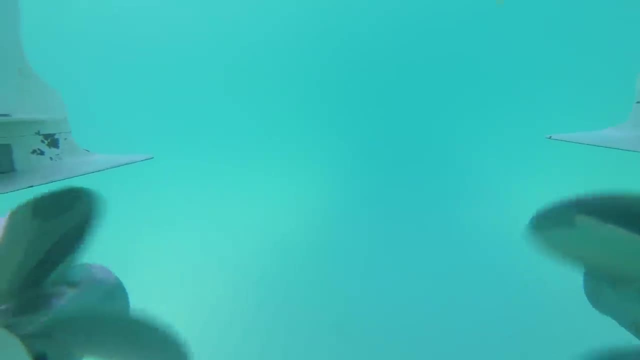 the boat weighs almost 2 000 pounds more, And this could be a conservative number, depending on the situation. That prop that was spinning, let's say 5800, is now only turning up 55, 54 or maybe only 5200 RPMs, which means that we are no longer propped out correctly. The more weight that the 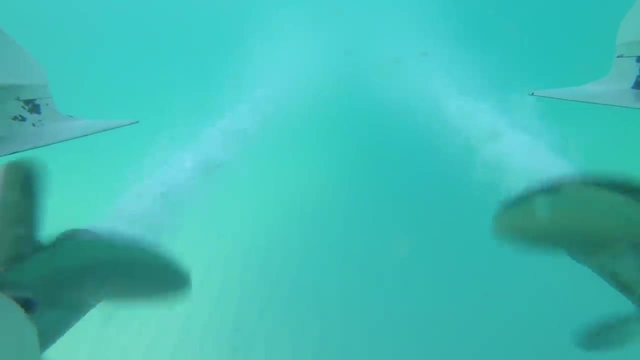 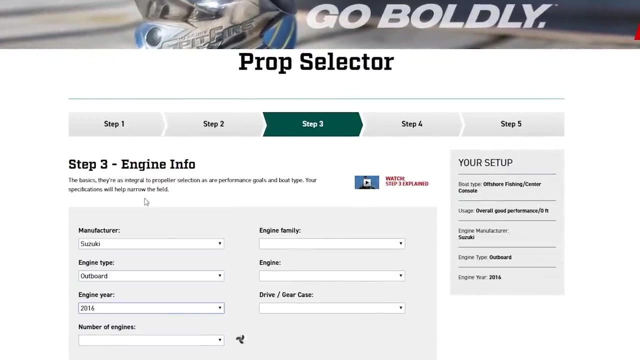 engine and the propeller has to push is ultimately what decides what prop we should use. We can pick a prop based on the recommended propeller from the factory or manufacturer of the boat. We can the previous prop that we were running in a repower situation or for just trying. 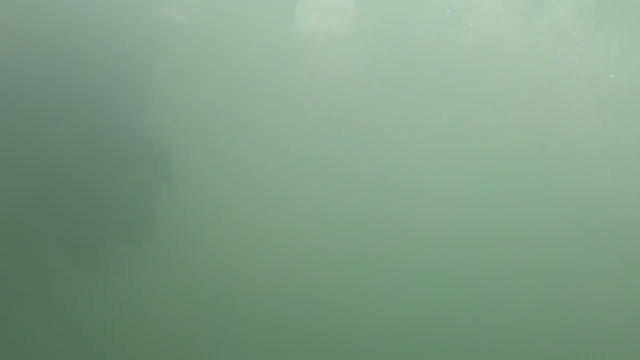 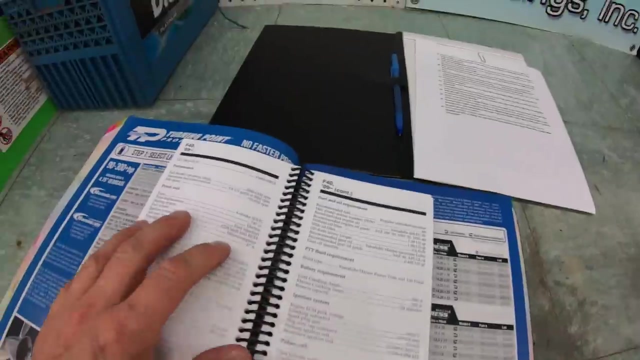 We'll install the prop and take the boat out for a test drive to try it. Let's say we have a 15 inch diameter prop with a 15 pitch, Our engine rpm range is 5000 to 6000 rpms and we've got close to the right amount of weight on board that we will normally have. 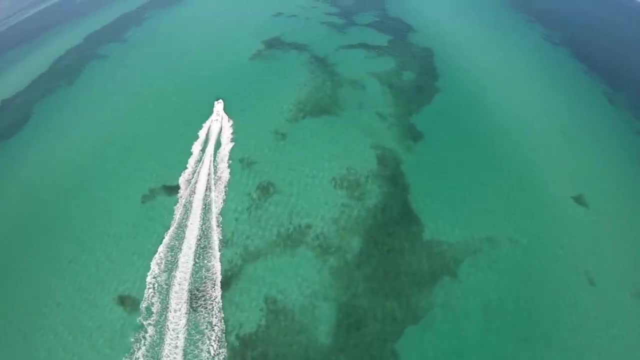 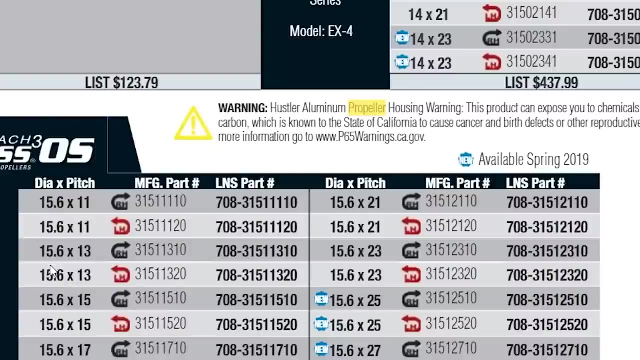 At wide open throttle our engine turns 6300 rpms and is hitting the rev limiter. This means that our prop is too small and isn't big enough to push the weight of the boat. So we can change out that prop and put on one with, say, a 15.5 inch diameter and a pitch of 23.. 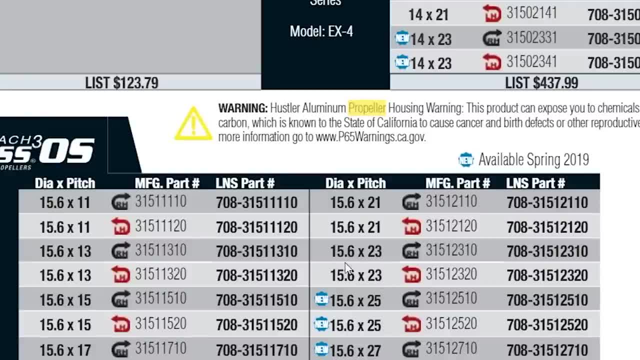 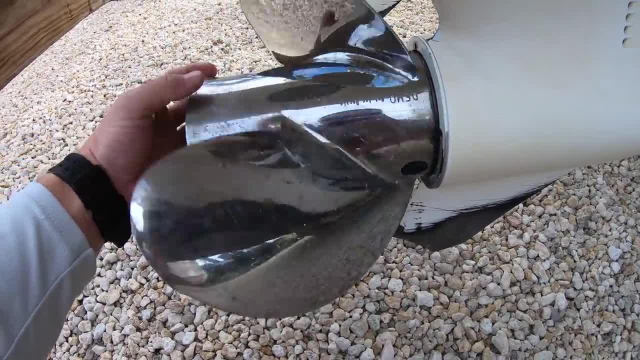 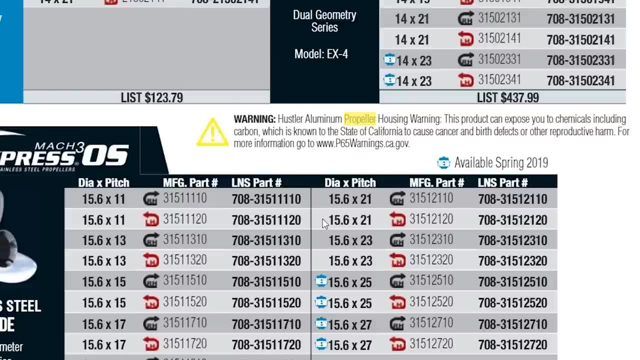 So after taking the boat back out this time, we only turned up to 5400 rpms. Now the prop is too big Given these numbers. we can keep that diameter and go back down to the 21 pitch and we will be looking at getting roughly 58 to 5900 rpms, which means that we have 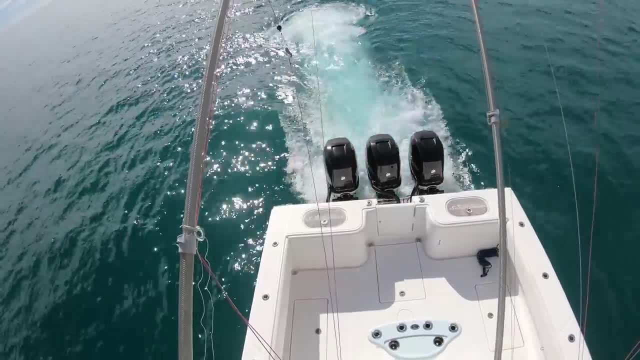 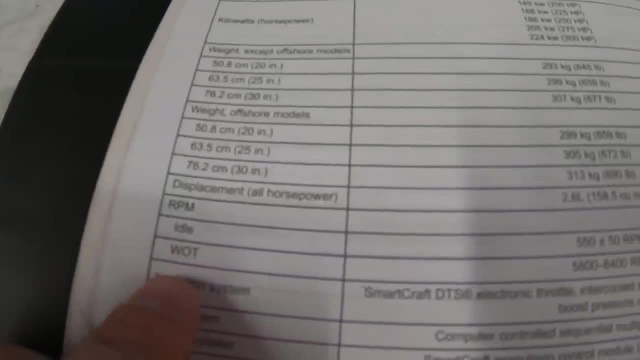 prop to use. We need to talk about trimming up. during this process, though Normally you won't have the boat fully loaded when propping it out, It's best to prop it out towards the top end of the rpm range without trimming the engine. We want to be able to add some trim to the engine. 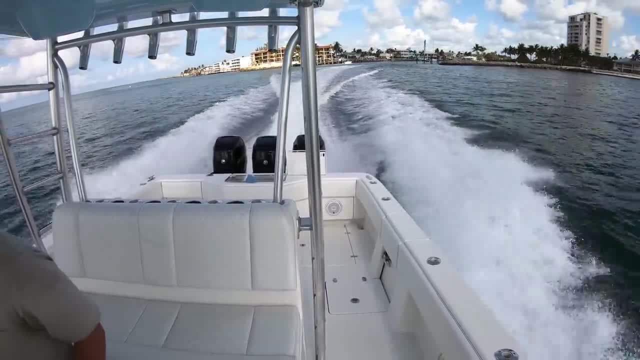 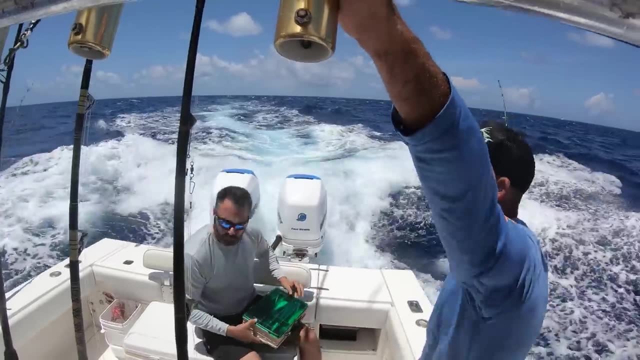 and come really close to hitting the rev limiter under these conditions. That is because whenever we load the boat up and take it out under normal conditions there will still be some room to add some trim at wide open throttle and have the rpms come all the way up. 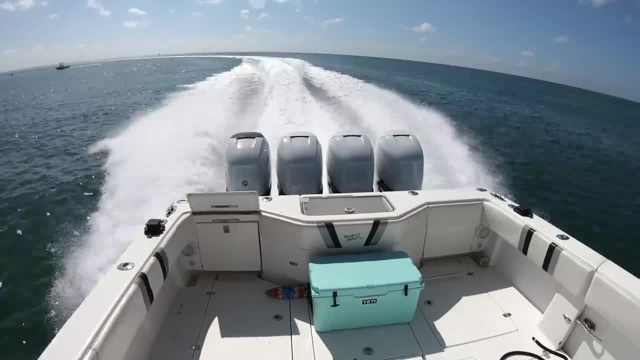 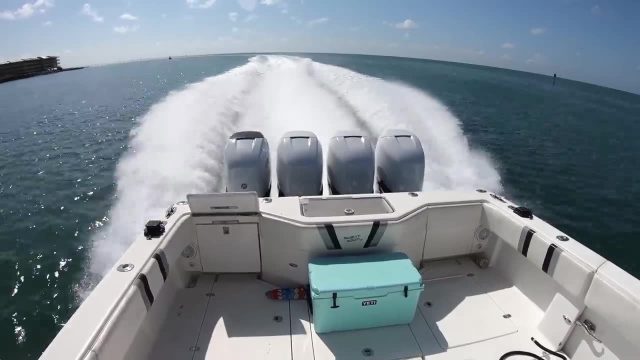 To the top end of the rpm range. if we have to trim up the engine to get to the top of the range, then after we load the boat we won't be able to get to the top of the range because of the weight that has been added to the boat. Now that you know how to prop out your boat. 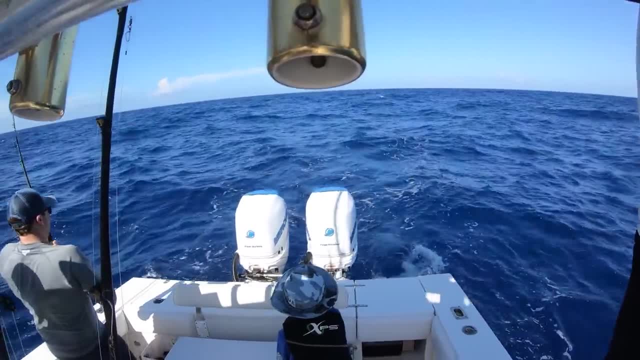 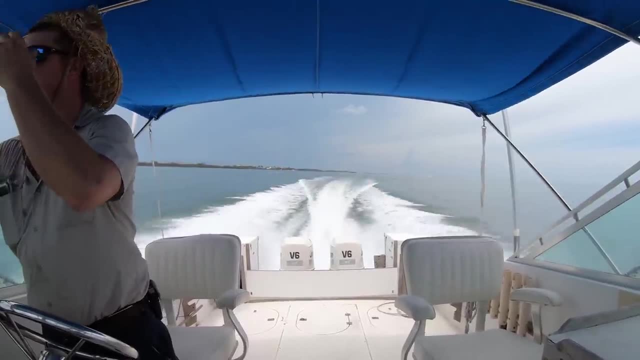 let us know about your experience in the comments below. Make sure to include a hashtag: clean boat for the contest prize. Follow us on instagram and let's talk about what having the right prop means for your wallet. Running the correct prop is going to save you some money because it. 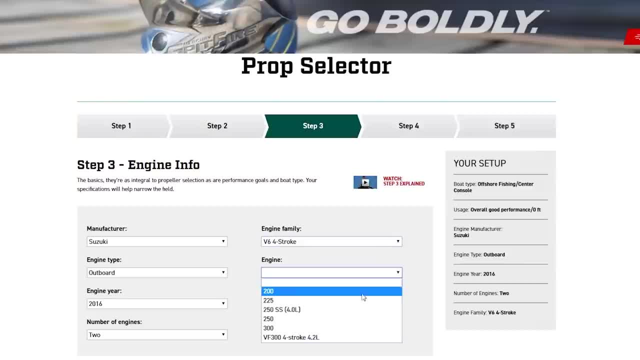 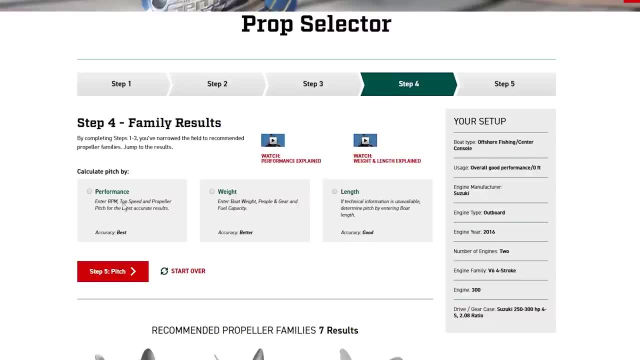 improves your mid-range cruising performance If running a small prop, you'll burn more fuel running higher rpms just to stay on plane at a good speed. Running too big of a prop means that you'll never hit wide open throttle and that will lead to carbon buildup along with